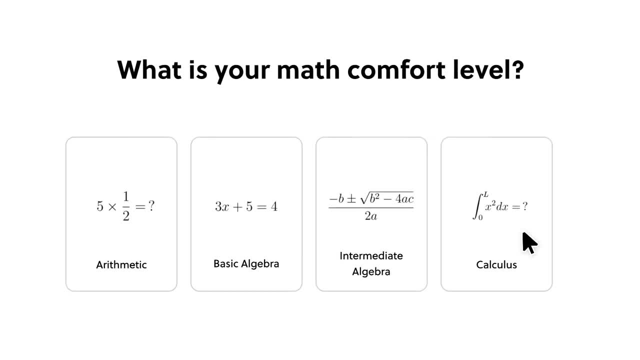 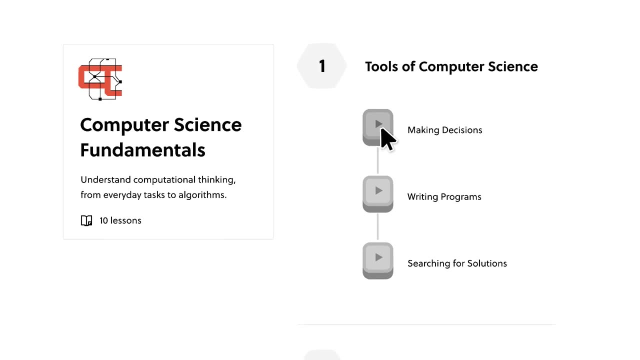 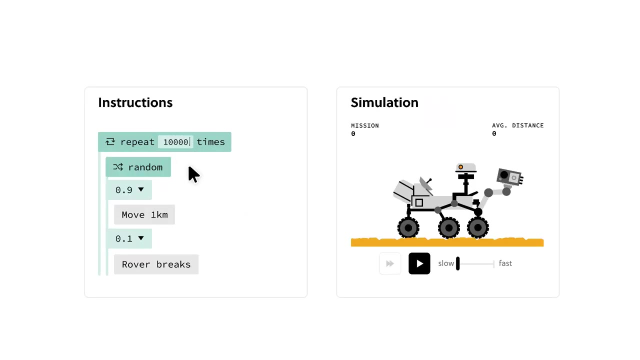 our sponsor, Brilliant. Brilliant is an online learning platform with over 60 different courses covering a variety of different topics in STEM, such as science, computer science and programming, as well as data science. I've personally had an absolute blast with the math courses it offers, as well as the courses it offers in physics. 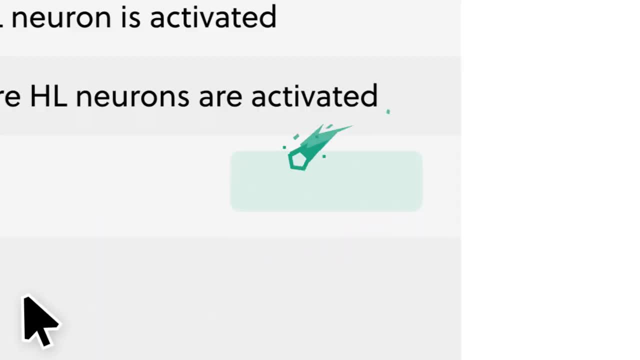 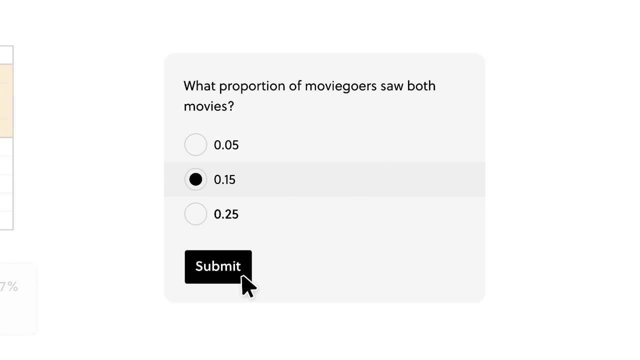 I've recently been looking at the quantum objects course, which I am just about to start playing around with this week. actually, One of the greatest things about Brilliant is its ability to teach you by playing. It gives you a really powerful way to learn by doing, which I find. 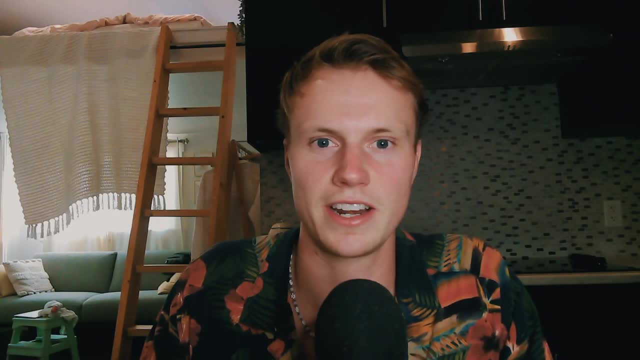 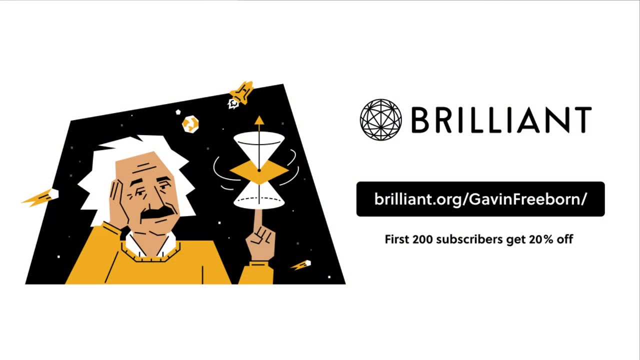 personally to be a huge help, and this is where Brilliant just stands out and stands well above the competition. To try everything Brilliant has to offer for free for a full 30 days, visit brilliantorg, slash gavin freeborn. The first 200 of you will get a 20%. 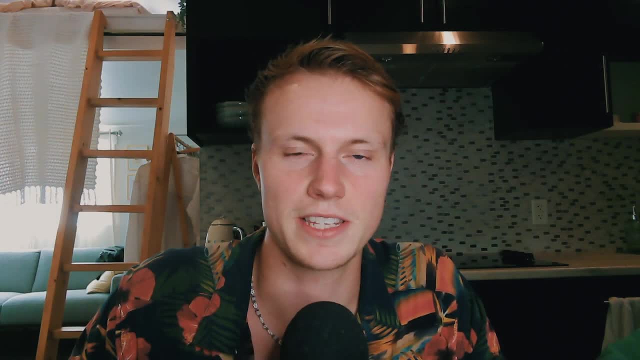 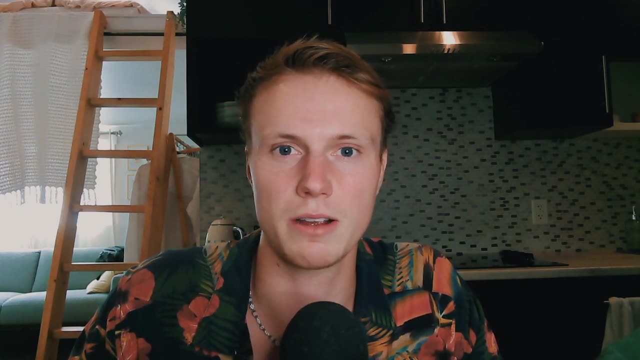 Brilliant's premium annual subscription. And finally, I'll be using some examples from an existing talk out there on YouTube. I'll have it linked down in the description. Very great video. highly recommend it. if any of what I talk about today interests you, He gives a really good. 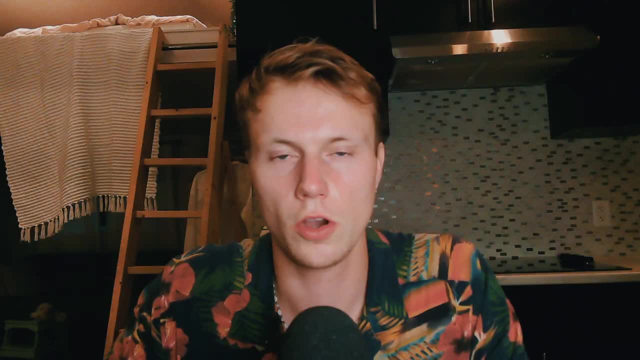 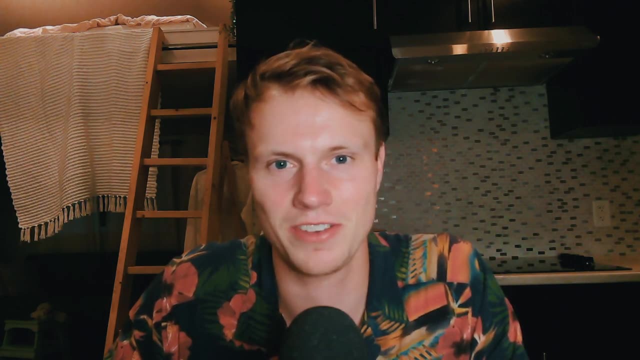 overview of the language, as well as what makes Haskell unique. Oh, and really quick. I just wanted to add a mention that I did use simplified solutions to some of this, so don't worry if some of my code looks a little long. I did that intentionally, because I found it just easier to. 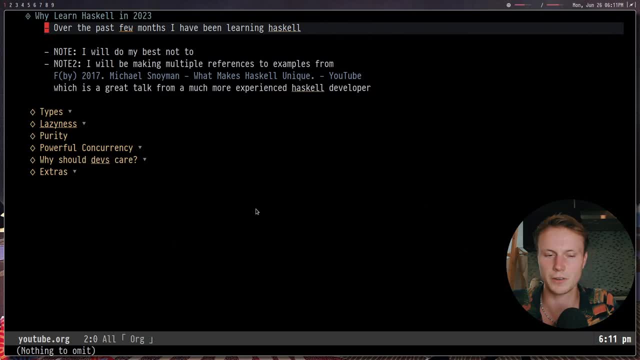 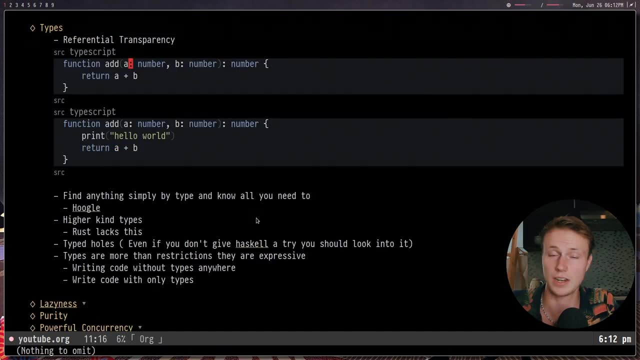 reason about. for those of you that are probably new to the channel, I'm going to be talking about newer to the language, So let's go ahead and dig into this. So first of all, here are the notes from above. Now let's first dig into the types. Types are a very important part of Haskell. Haskell is 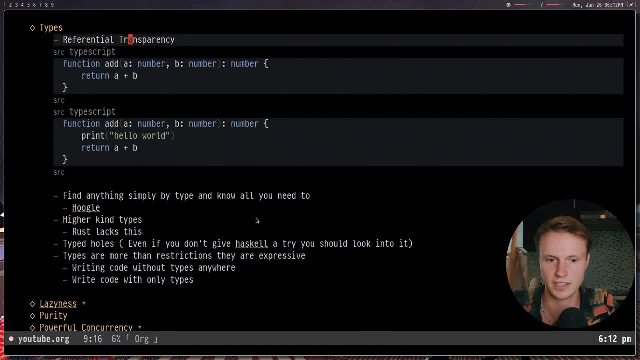 a statically typed language and so, as a result, since it is statically typed, everything has to have a type. There is no switching of types, so what is once a number cannot become a string later. So the first thing that the type system in Haskell brings to us is referential transparency. So in 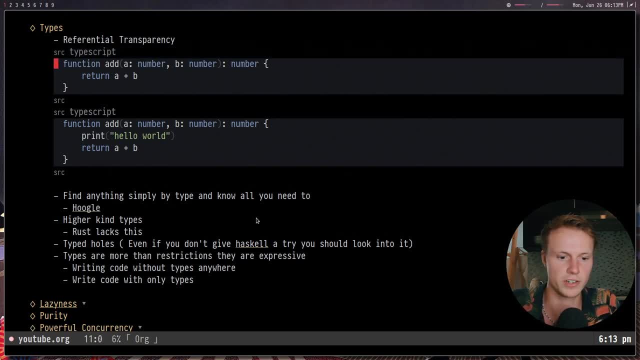 TypeScript and this is just kind of like I said before I made up the type system. in Haskell You can have a function called add. You can add a and b, where a and b are both numbers, and return a number, just like this. Now what we could do is we could print hello before we return the number. 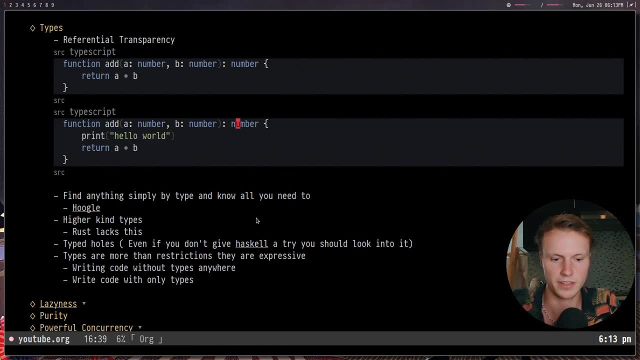 However, note that this does not change the type signature. So even though we say we are returning a number, there's no indication that we printed this data. In addition, we could do really anything in here and there's no real transparency showing that this has happened. Now in Haskell to do the 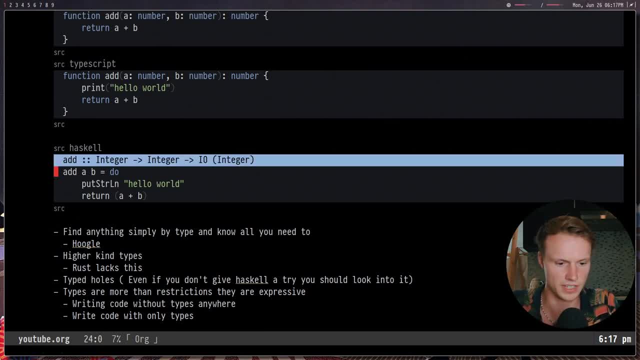 same thing. we could do this right here would be the Haskell equivalent. So, as you can see, we make a little type declaration which basically says: we take an int, we take an int and we return an integer wrapped in an IO. Now, an IO basically means that we are going to be doing some IO operation. 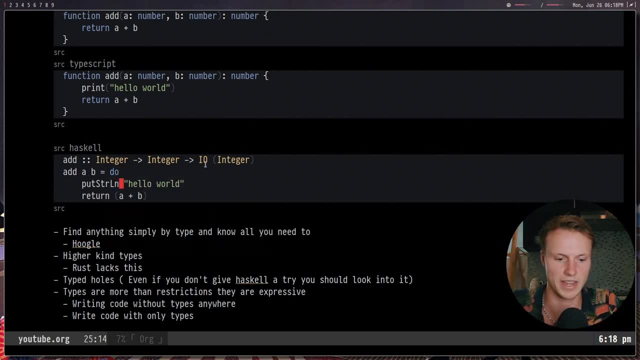 and so that is what is basically happening here. We are transparently showing that we had to do some sort of IO operation and then we wrap our return in that. So this basically gives us what I was referring to before as referential transparency. 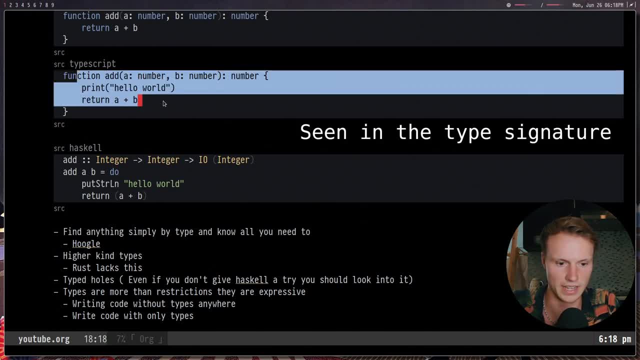 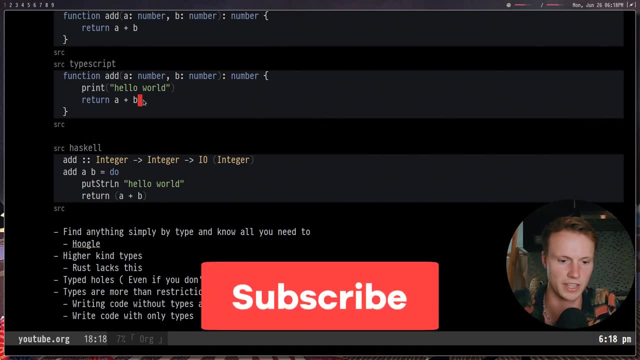 There is a clear IO operation that had to take place, whereas that was not necessary here when we used our fake version of TypeScript, But I'm sure you guys that are familiar with pretty much any other language can think of an equivalent here. that is not really possible with Haskell. 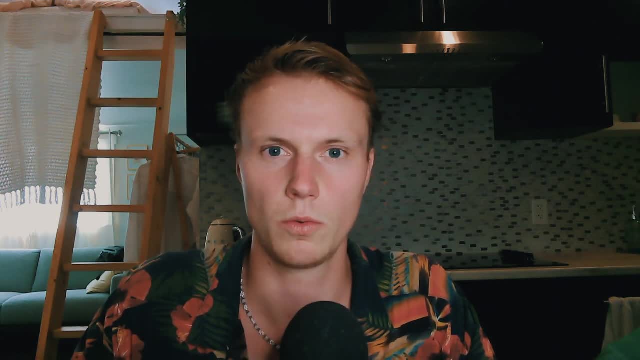 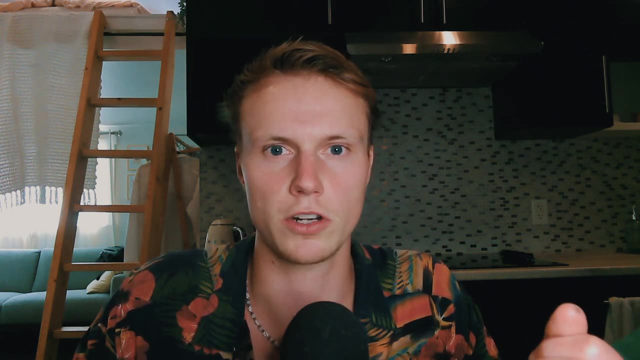 So why does this matter? Why do we want referential transparency? Well, a big reason for this is the ability to debug code and basically being able to control these effects. For anyone that's worked on code that has a whole lot of IO operations, it's best to keep the IO operation in the 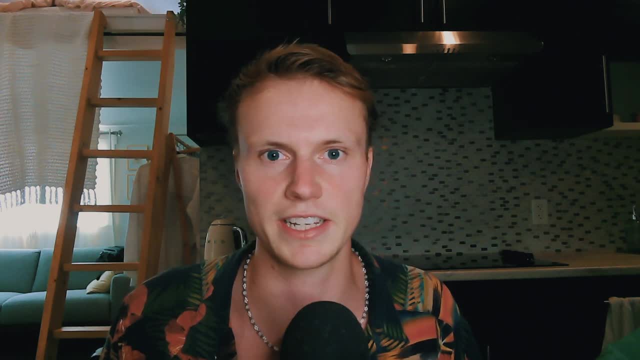 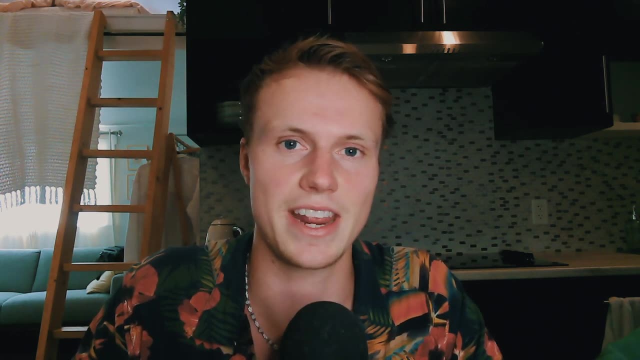 same place, and the last thing you want is code that is secretly doing an IO operation. Often, this sort of situation results in very buggy code and a lot of issues and a huge headache when it comes to debugging. And so what do we get out of this? Well, we get the ability to do very powerful 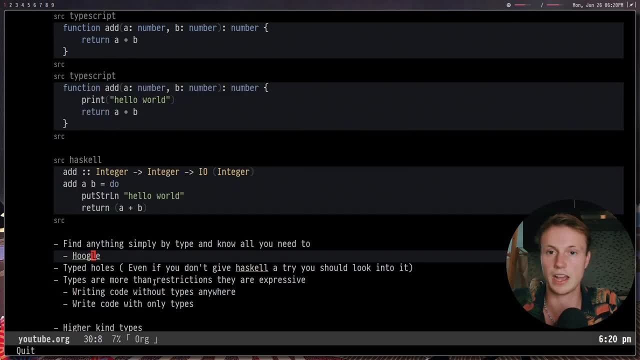 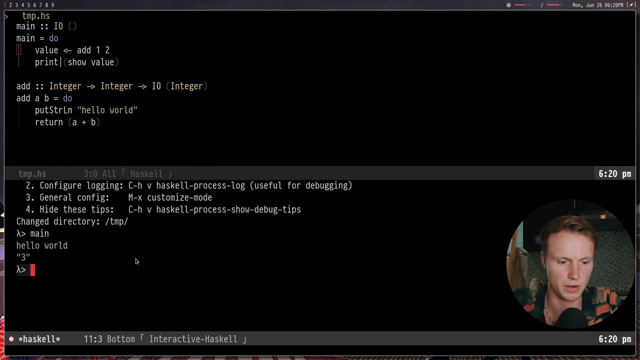 searches. So we could use something called Hoogle, which allows us to basically look up something based on the type signature as well as typed holes. So, for example of the typed holes, let's just go to IO. I just used this while I was writing my simple example before. Now, if I just open up a REPL, right. 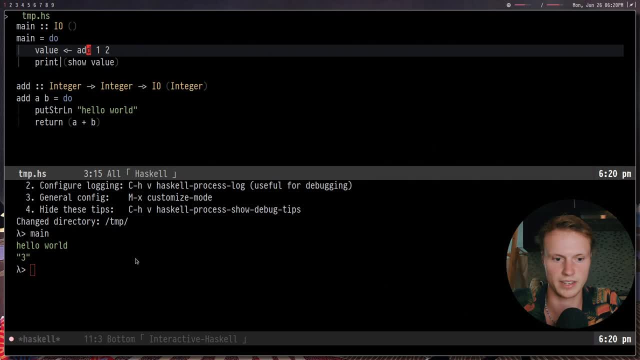 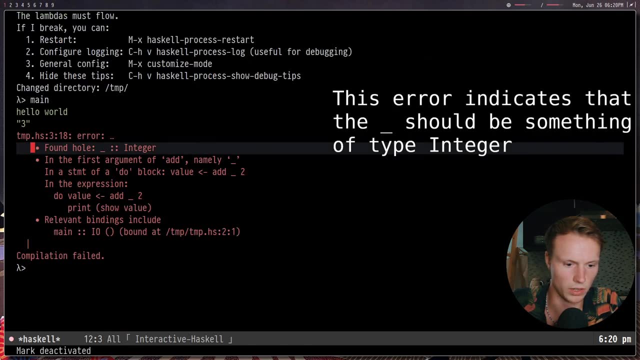 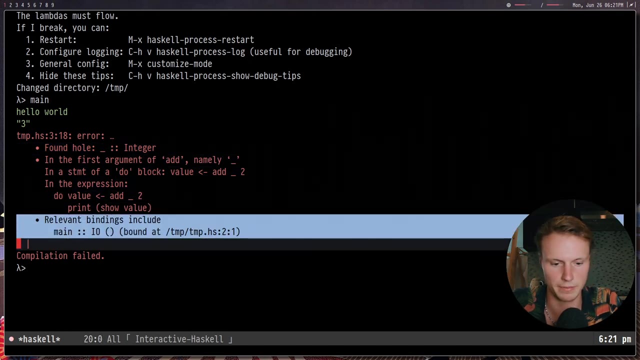 here I can actually sort of play around with things. So if I delete that one and replace it with an underscore- and I evaluate that we will get a hole here, Now we can get information on the hole, such as an integer, and it will try and find relevant bindings In this case. that's not a thing. 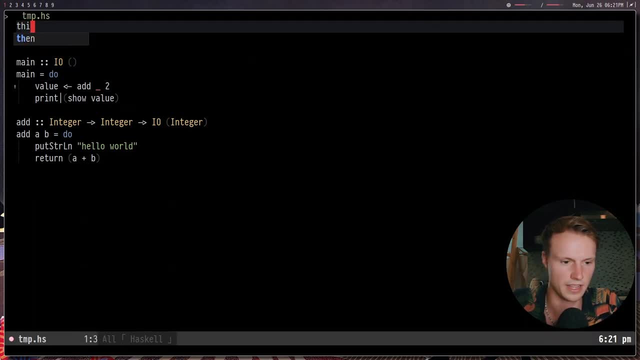 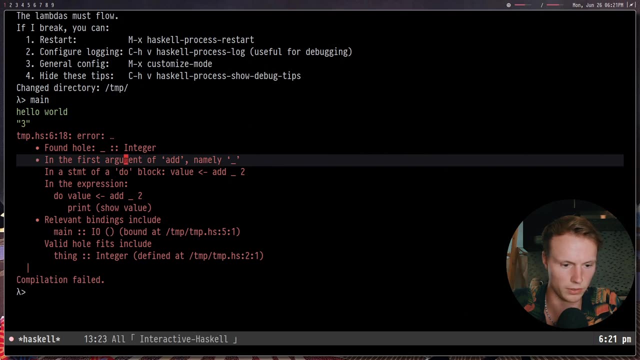 we don't have any useful ones. but let's go ahead and make a thing of type integer And if we load that and open up the REPL we will get a type hole. It can't find it and it will look for relevant things that fit our type of integer. A valid hole fitting includes a thing, So that is. 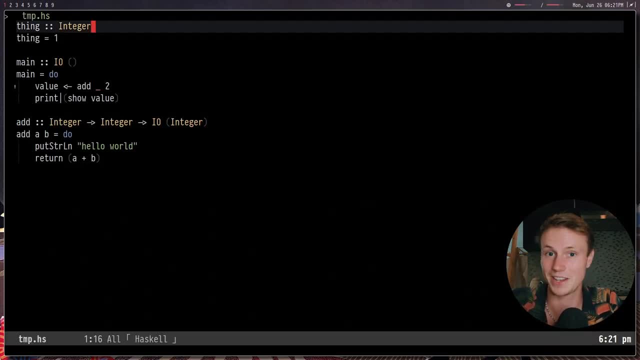 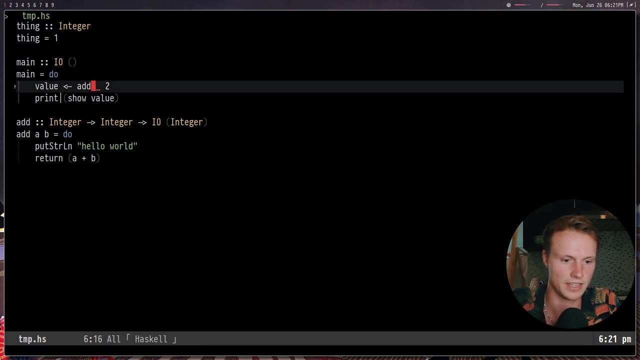 our thing from right here, So you can kind of get Haskell to basically write itself. It sounds really silly in this case. this is obviously a simple example, but a good example would be: let's say instead: we have thing and we don't know what we want to do here. All right, so now we have a hole. 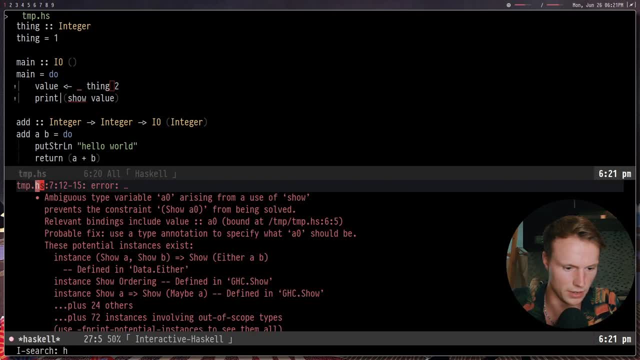 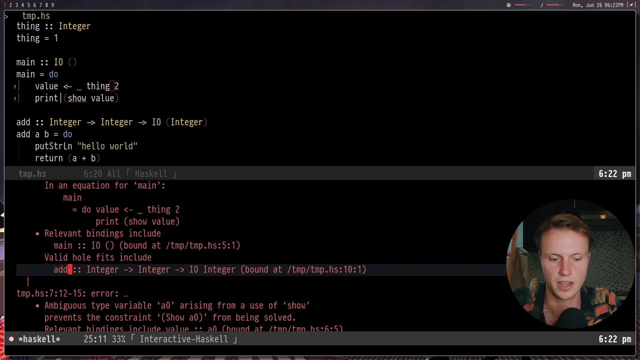 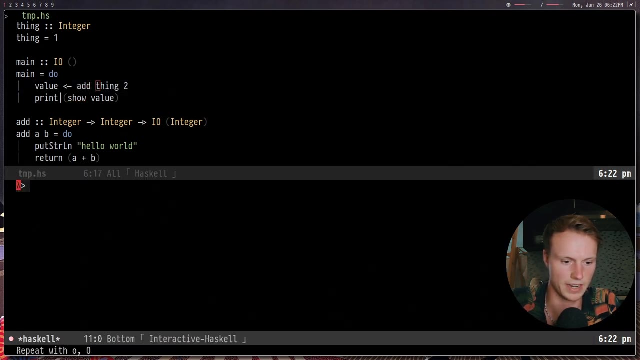 fitting and we want to see what our add was. So if we evaluate that and we take a look, we will see valid hole fitting includes add. So there we go. there's a very simple example of how you can use this referential transparency to actually find things that solve your use case. Add here: load. 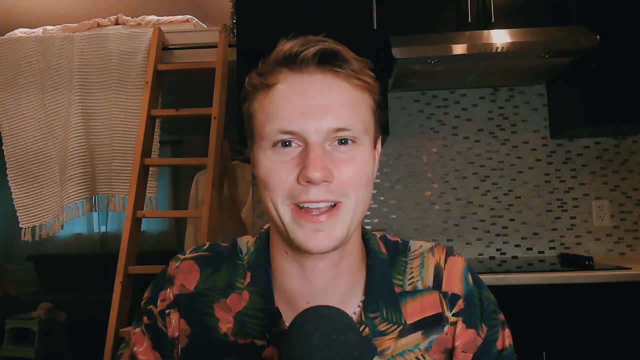 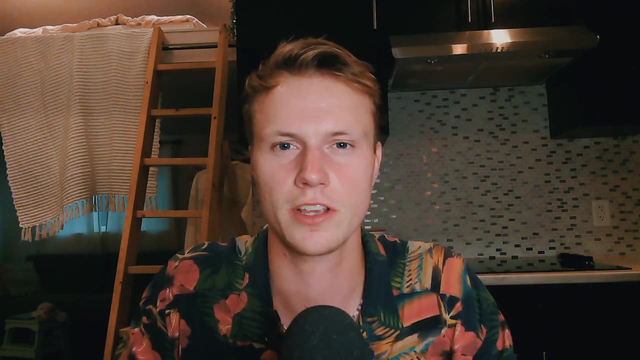 that again and there are no errors anymore, And then we could just do main runs perfectly fine. Now, really quick, I want to talk about type classes. Type classes are probably one of the big things that kind of differentiate Haskell from a lot of other languages. These days there is a somewhat equivalent concept called interfaces, Although interfaces aren't really quite as powerful in a lot of languages, mostly because they lack higher kind of types. Languages like Rust, Java, a bunch of other different languages lack this concept, which is basically a way to abstract over a type constructor. Not really going to go into that. 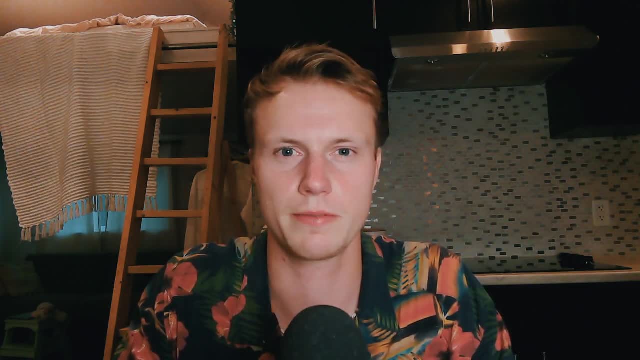 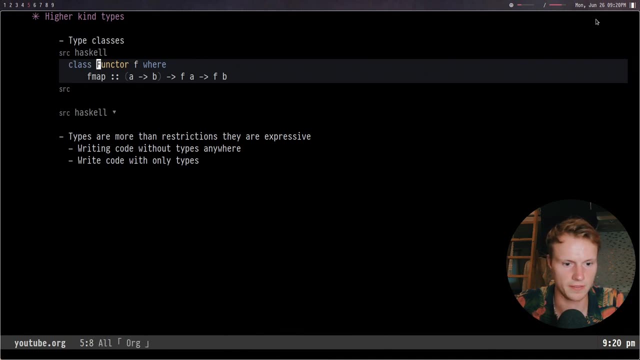 but let's just go ahead and look at an example and you can kind of sort of get the concept of what I'm talking about. So here we have a type class called functor Now, but what we're saying here is that we're going to use a type class of the name functor. In this case it is f. so when we refer to 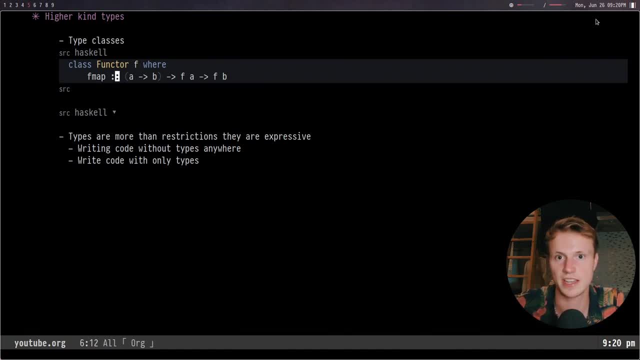 f. it is some functor where fmap- so that's the name of the function- has the type of a function that takes an a and turns it into a b, and then it also takes a second argument of a functor a and then it returns another functor of b. So basically we have a way to. if say this was a list, we could basically 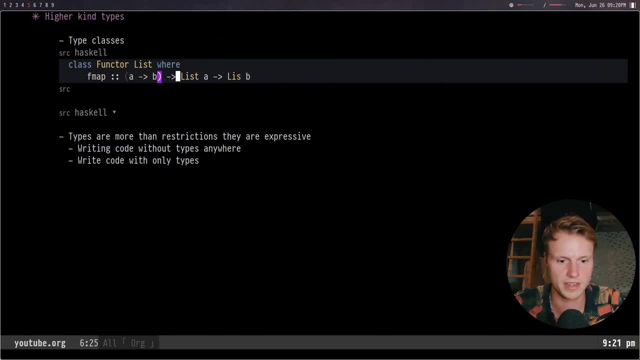 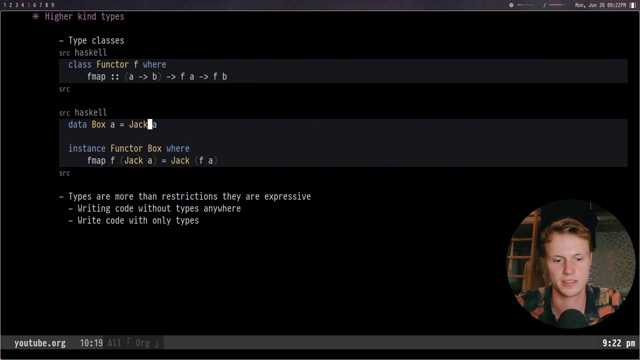 think of this as f could be a list and it takes a function of a to b, A and it returns a list of b. That's basically the concept of the type class. Now we can implement this just like this. So I made a data type of box Jack is a way to construct a box Jack in a box. 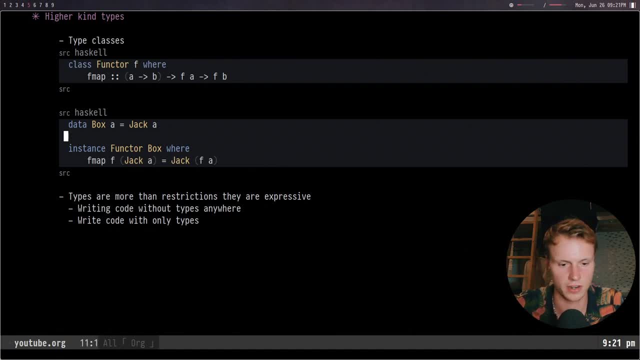 You can't. you kind of get the idea. maybe This is kind of the type constructor of of a box is jack. Now, in order to map over it, all we need to do is create an instance of a functor box where we can map a function of f over a jack of a by simply applying the 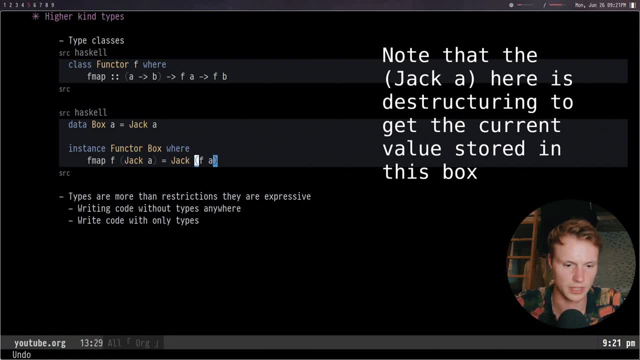 function f to a and then wrapping it in jack. This is actually probably the best way to describe it is basically just a list and then if we wanted to do it like this. So basically, what we're saying is we're implementing some way where we can apply a function to our container, which, in this case, I'm 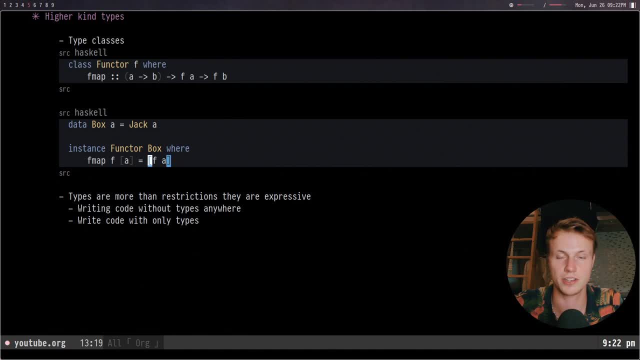 treating it as if it was a list, but it's not actually a list, and the best way to implement that is to simply apply the function to the contents of our container. This is kind of where we're going to be doing this, So I'm just going to go ahead and just do a little bit of 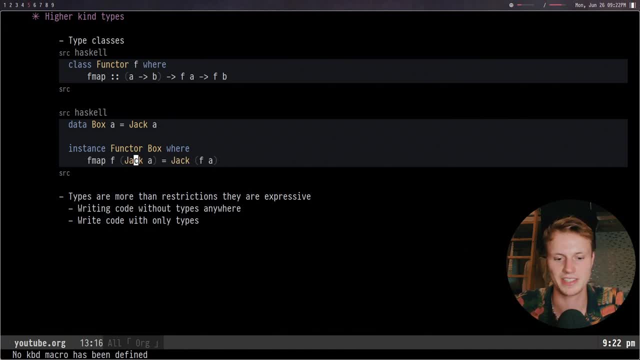 abstract over these type constructors, just like this. Now, sorry if in advance, if that's a little complicated. The great thing about this is that you don't really need to go too deep into this, right out of the gate You can play around with it and then you can kind of learn this as you go. 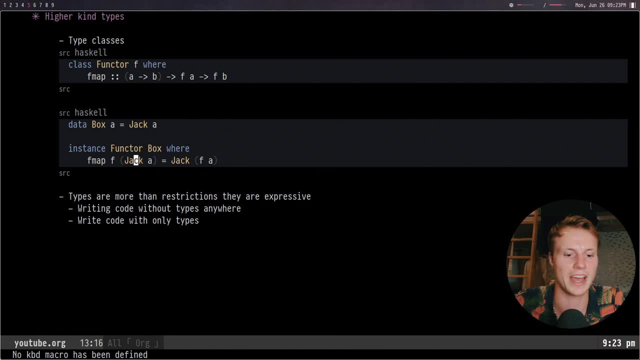 It'll make a lot more sense once you've kind of played around with it. I'm not super experienced at explaining this either, so I'm probably a very poor teacher at this part of the code. Hopefully in the future, if I'm a bit better at it, I'll try and explain type classes a bit better and 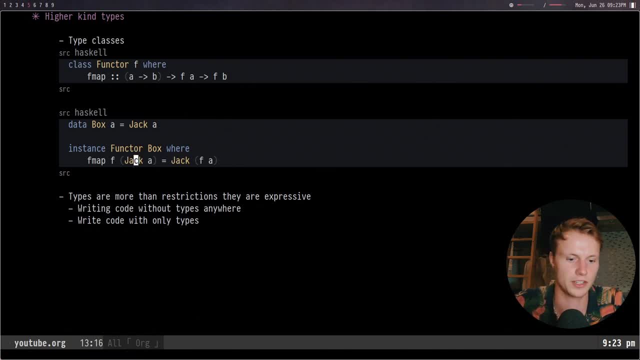 then I'll just go ahead and show you how to do it. So the great thing with type classes is that we get these higher kind of types, which allows us to abstract over things like a constructor for a type which is extremely powerful and gives us a lot more flexibility than we'd get in other languages. 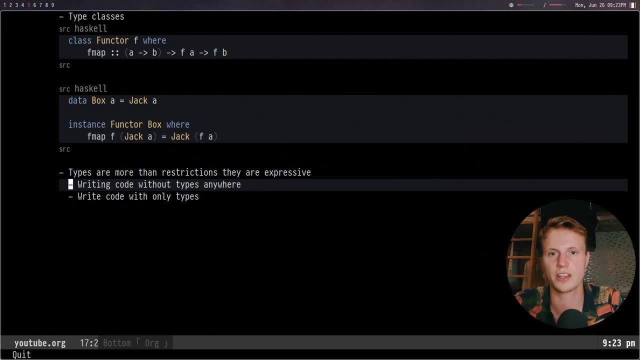 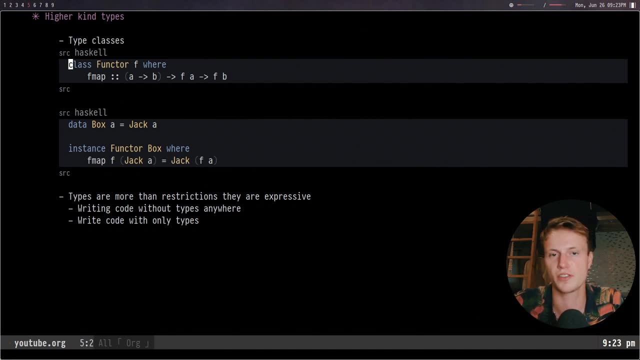 out there with a simple interface. Now, a key thing I wanted to mention is that types are not a restriction. They are a way to be expressive. These are basically a really powerful way to implement a DSL, if you will, or a domain specific language, where you can make a type class that kind. 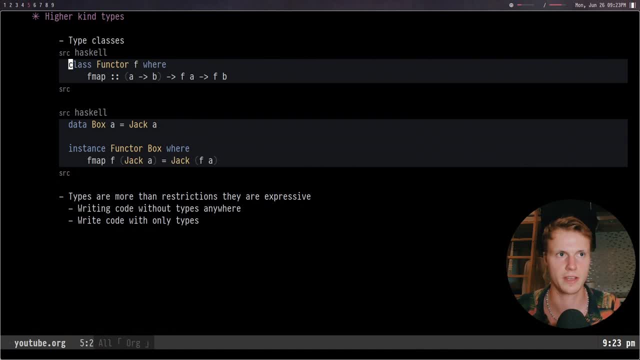 of fits your needs and implement certain things, So you can kind of use polymorphism to sort of make it all look the same even if you're working with a bunch of different types, and that's super powerful. Probably a really good example of this is parser combinator libraries. I'll link some down below that you guys can look at All over. 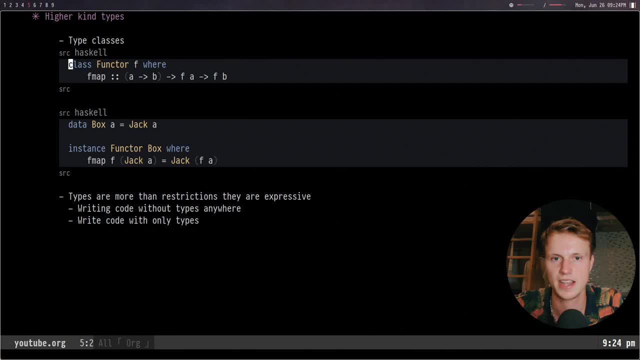 the place it's used for describing endpoints in a server. It's really powerful and it allows for very concise code. Obviously, for newcomers it's a little scary at first, but once you kind of learn to read the syntax of Haskell, it becomes a whole lot easier. Now I wanted to really quickly dig. 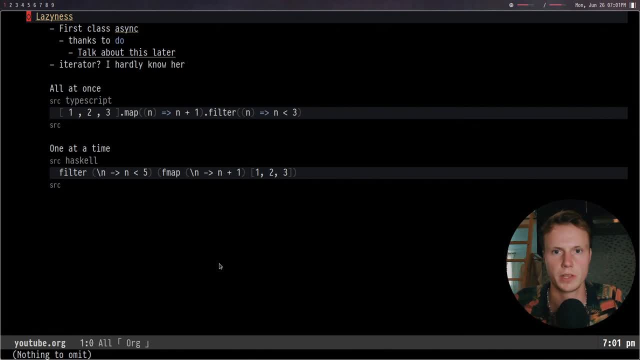 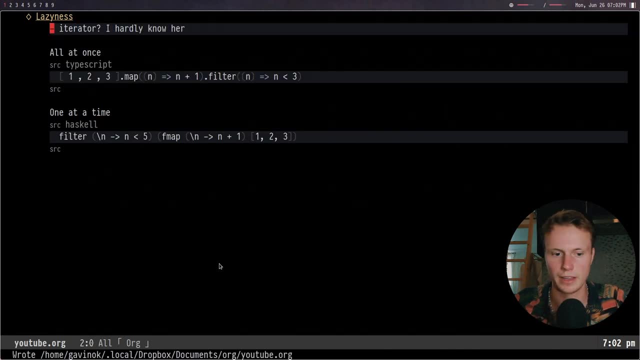 into laziness. I don't want to go too deep into it because it mixes in with a lot of the other stuff we'll talk about later. I just kind of want to quickly introduce it, So we'll go ahead and skip over this part for now, and we'll talk about that later. Now, what I wanted to talk a bit about is: 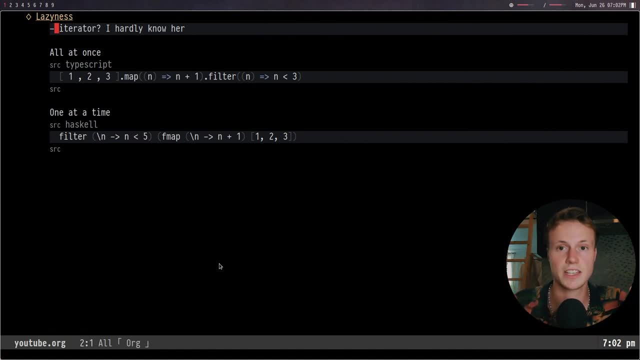 how laziness allows us to avoid the common use case of iterators. So iterators allow us to do something like this, where we can take some sort of a collection, we can map over them. So for each element in there we will add one to it and then we will filter it down to three. Now, if you're 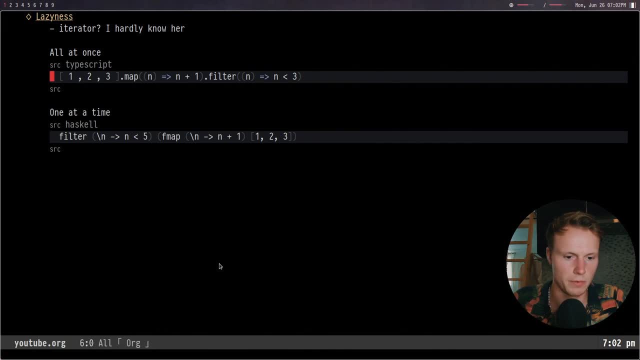 using Haskell, you can filter it down to three. Now how this would work in regular programming is: we would, individually, we'd go through each of these steps all at once. So we would do one, we would take one, we would add one, we would take two, we'd add one again, we'd take three and 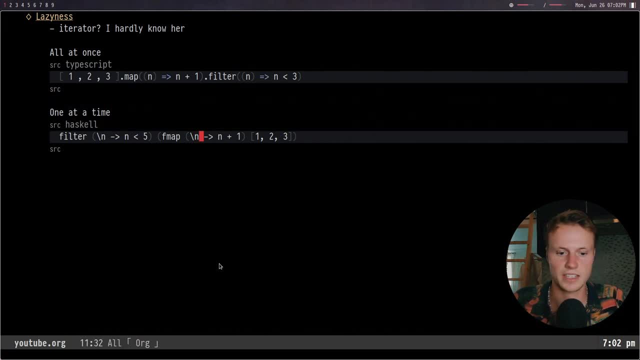 we'd add one again and then we would pass it to the filter Now with Haskell, since it's lazy. it will only do work when it needs to. So instead of doing all of this at once, it will only get the final result when it is required. So, in theory, 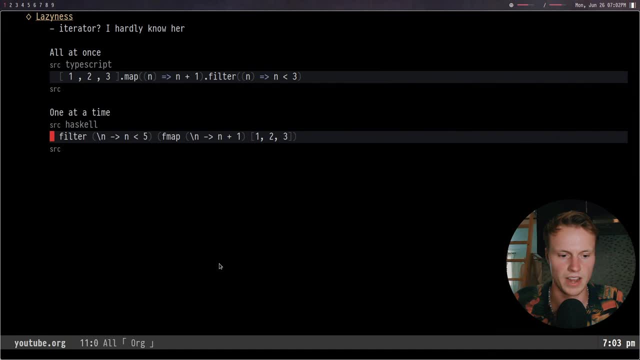 if you only needed the first element, then it will only go until we find something that passes the filter. So it'll add one to one, it will filter it is less than five, and then it would get that first result. Now, a lot of languages, like Rust, for example, implement iterators and a lot of 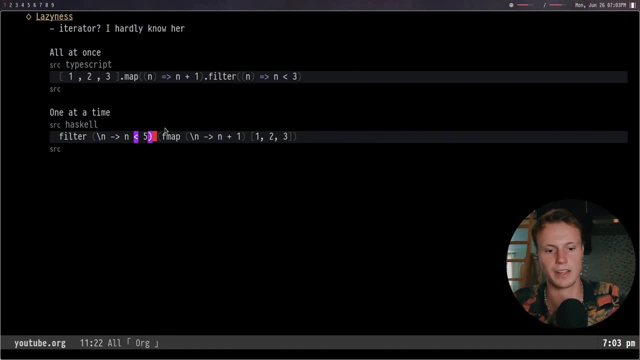 other languages do this to kind of work around this, But with Haskell, since the language is lazy and it does this for everything in the language, you can avoid this overhead and you can get some really powerful features as a result. Now, this is only possible because of the fact that 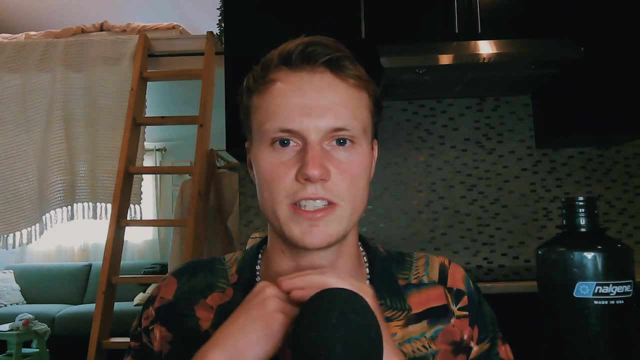 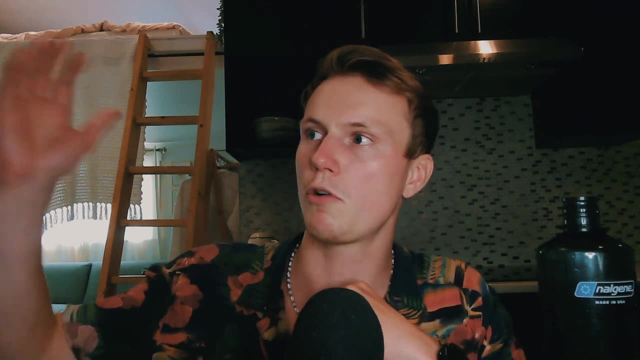 Haskell is a pure language, So I want to talk a bit about concurrency. So let's think for a second. There are a bunch of different places that you could get data. For example, you could get it from a remote resource, Maybe say that remote resource takes some time to get to, and then you want to. 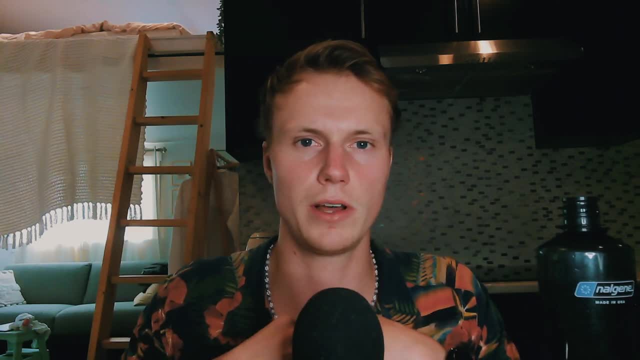 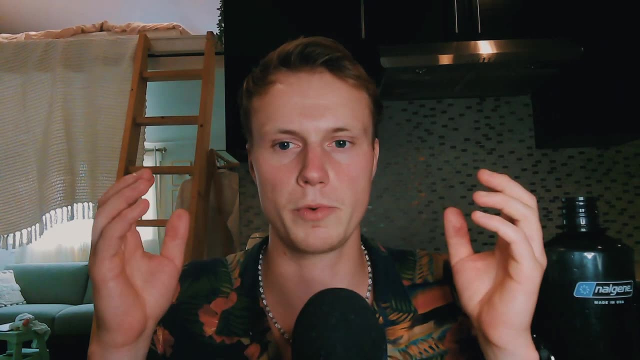 cache it, or maybe you want to store it in a database. Well, let's just say you have all three, or maybe you just have two. In this case we'll just use two, because it makes things easier for me. Say, for example, we've got a cached piece of data, or we have it in a remote and we don't really 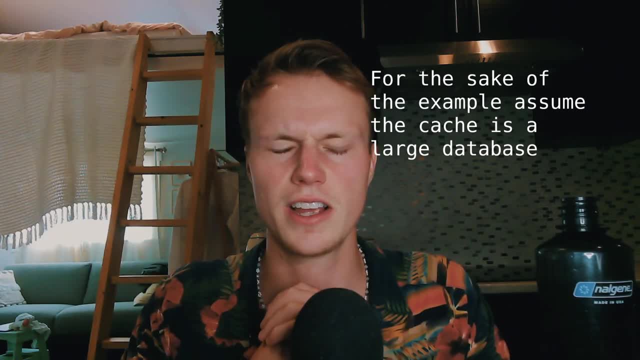 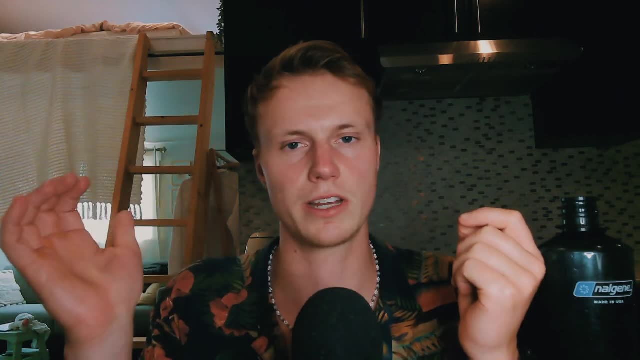 know which one's an option. Now one could be faster than the other, especially if, say, we have to do a big lookup. So in this case we want to kind of say, okay, look up here and look up here. I want to do both of those at the same time. Now this can get rather complex and you require 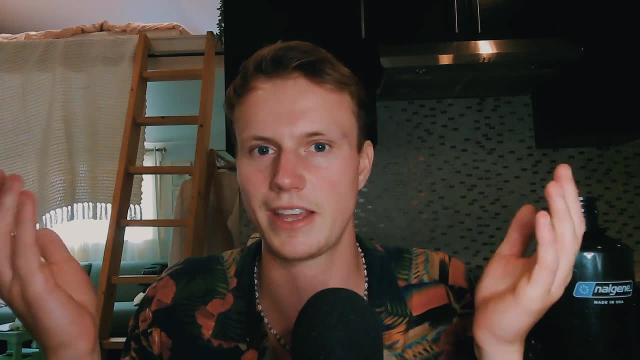 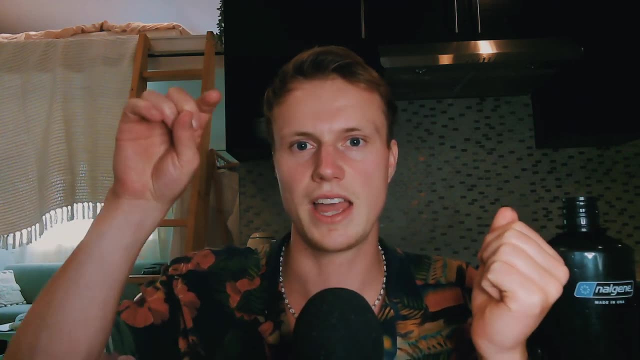 the ability to either cancel or- I guess you could run things to conclusion. but that kind of defeats the point. You just want to run two things concurrently and get the result. Now, in a lot of languages you'd have to execute these and have a edge case where you would cancel. 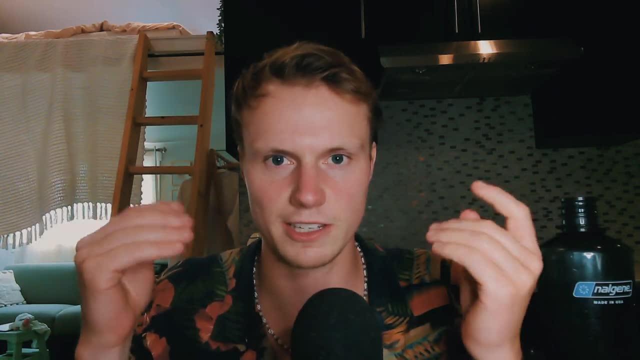 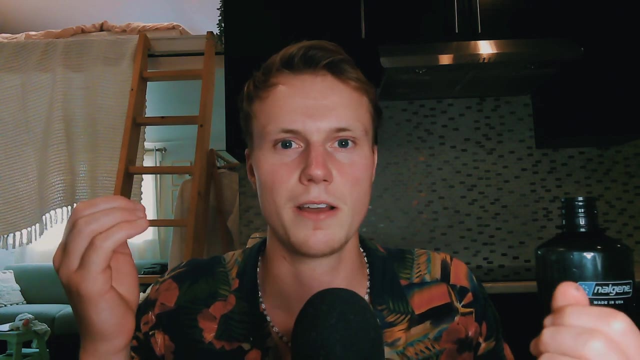 a thread, or maybe you would start another thread Now with ASCLE, since it's all lazy and this is all handled by the language itself. we only have a single function that will do this. Well, we have multiple, I'm sure, but the one that I know of is called race, and so here is the code. So you 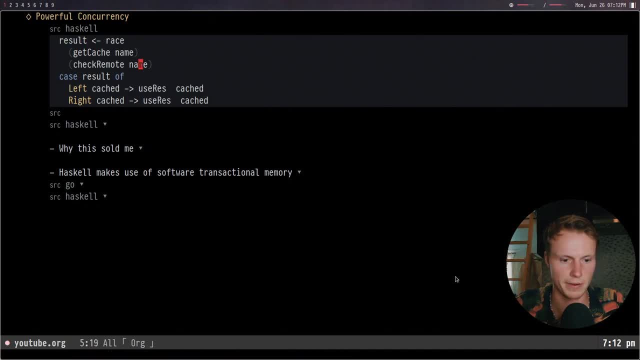 basically get a single result and we race between the get from cache and the get from remote. Now one could be faster than the other- it's hard to really know- and so this way we can kind of run them concurrently with each other. Then we finally get a result and we can go ahead and say: if it was. 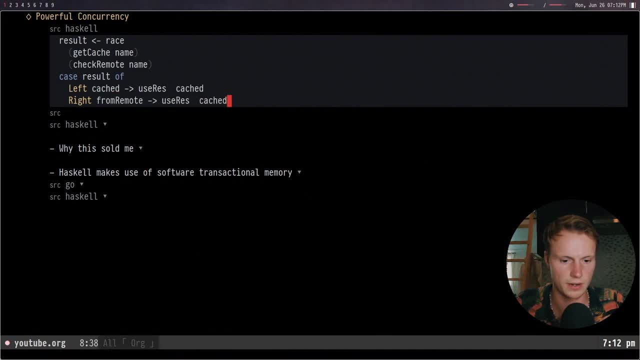 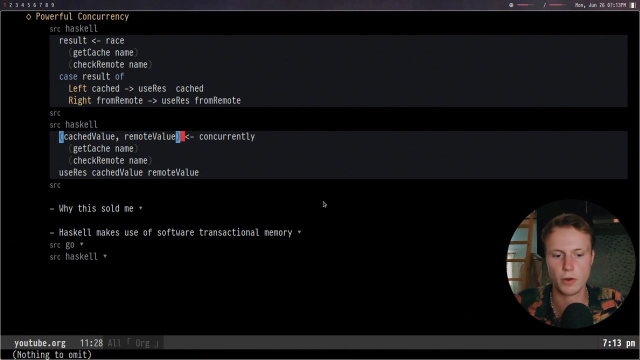 the left, then it was cached And this is, and then we will just run the function on whichever one we get. So this gives us a really simple way to kind of run two things and take the first result. Additionally, a probably more common use is that you want to run things concurrently. So say you got a cached result and a remote result. 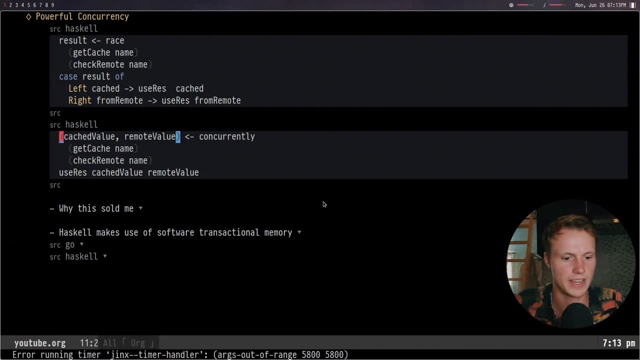 and you want to see if they're the same, Update the cache if it's out of date. So in that case you could do the same thing but you would use concurrently and then you would get back a tuple and you can use this tuple in your function instead of just getting the first result. Now I 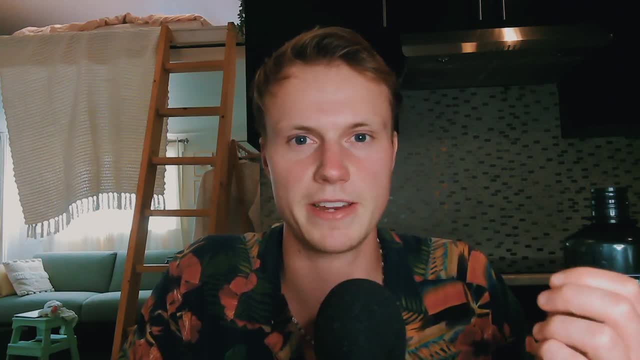 want to talk a bit about what we're going to do next. So we're going to go ahead and run this and then we'll get started. So let me just run this and show you guys why this was so important to me, that it convinced me to give Haskell a real try. 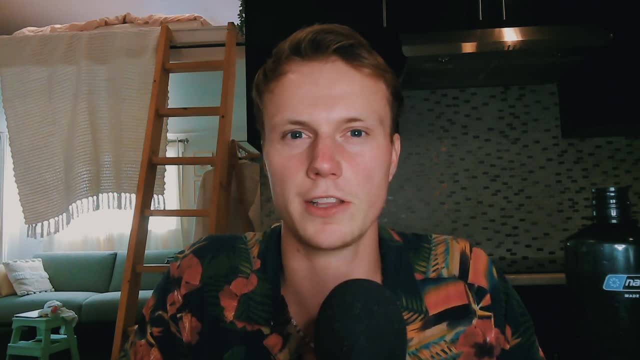 Now, the big reason for it is that I was working on a fairly large project with multiple developers all working on something that had basically two requirements: It needed to be able to handle a thousand users- about 10,000 requests- and it needed to be fault tolerant. It was going to consist of: 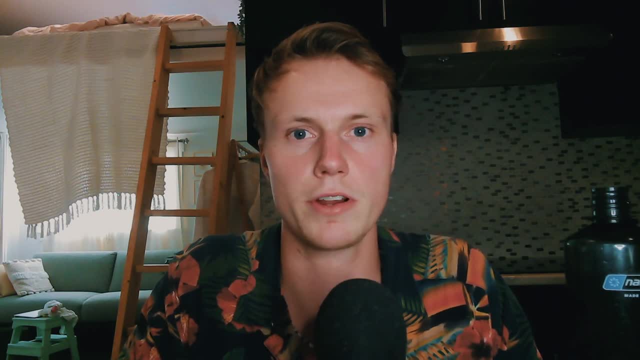 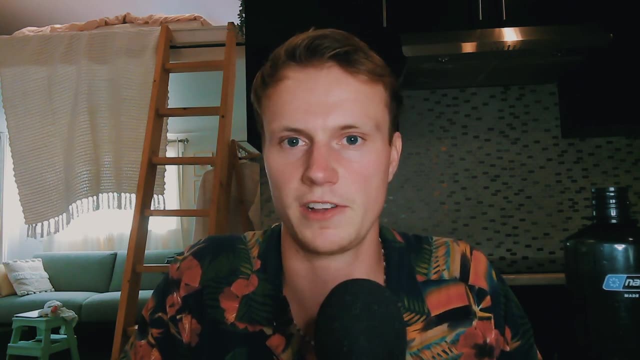 multiple microservices, and so, because of this, we needed a pretty powerful system that could handle a ton of concurrency, And so, at the time, the language that we just used was Go. Go is a perfectly fine use case, we thought, and which it is to some extent, and so it had some really powerful 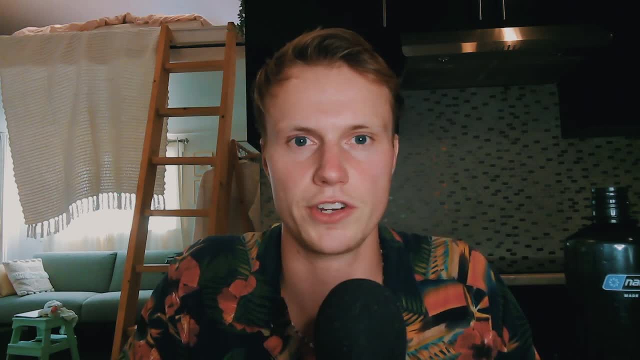 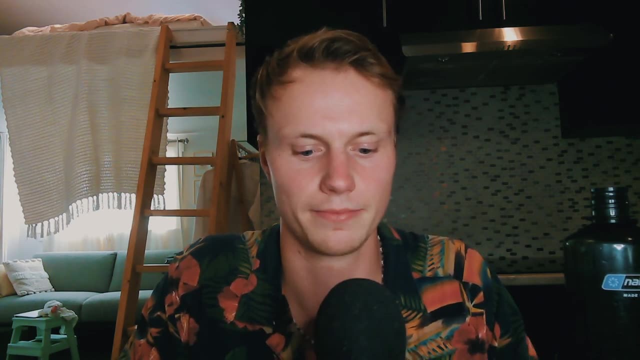 advantages in its concurrency model. but we ran into a few issues, and this is not purely the fault of Go. I'm not trying to make this a versus battle. I'm just kind of talking about a situation that I ran into. Something we ran into that became a major issue was the inexperience of some of the developers with working with concurrent code. Now, while this isn't a massive issue- and obviously code review is important, it made kind of debugging the code and making sure that everything was sound. there wasn't anything being passed to a closure that was going to be referenced later on. 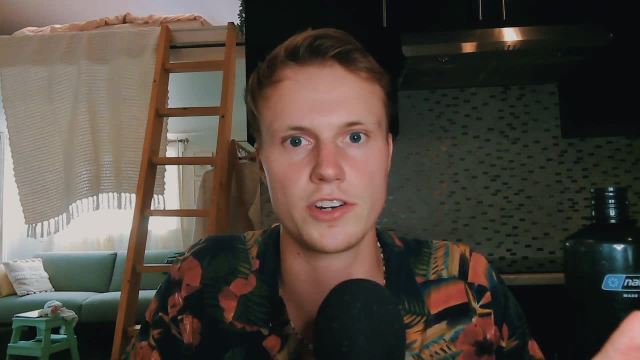 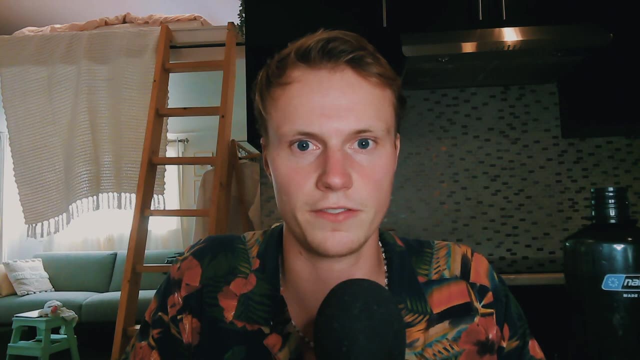 because that would kind of obviously mess with the ability to make things concurrent if you're sharing state between all these threads without locking or anything like that, And so, as a result, you end up to either lock when you're unsure of things or having to really abuse channels to the 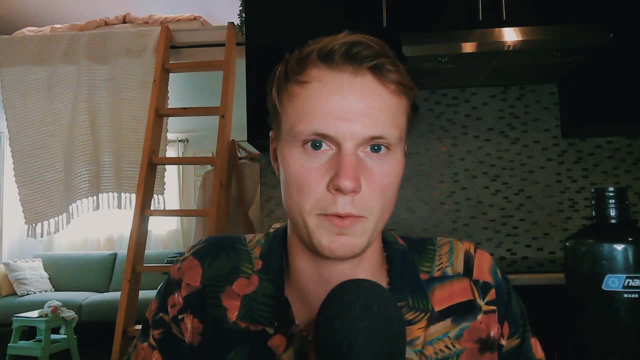 point that it got really messy- And this is kind of where we ran into our problems- was mostly because people would end up accidentally sharing information between different places or they wouldn't realize that something wasn't going to be constant. it was going to be referenced elsewhere. 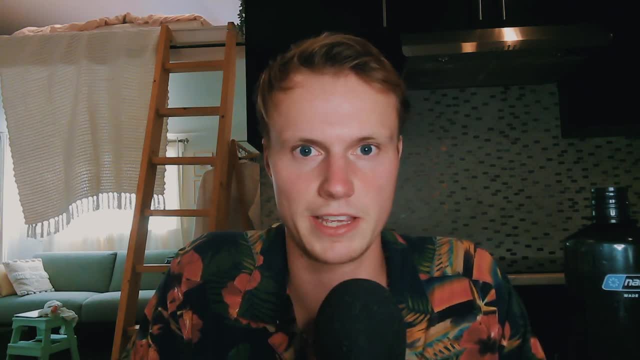 and so we couldn't count on it as staying the same, which is a really common thing that you end up doing. You can you try to count on things as being the same. that way, you aren't having to worry about locking all the time, but, as a result, things can get very messy And something we ran. 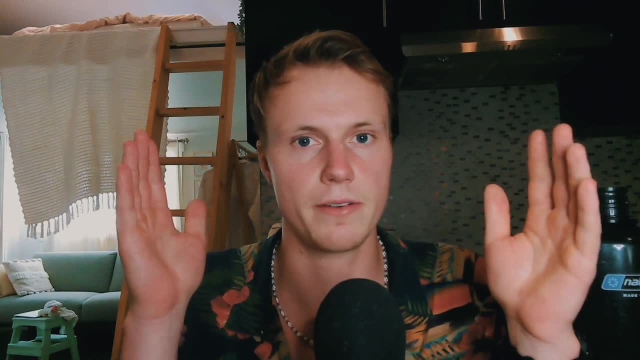 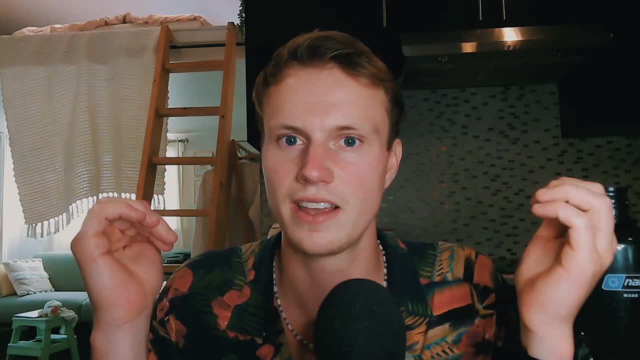 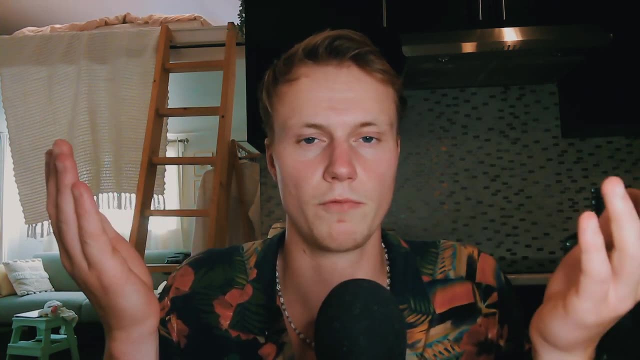 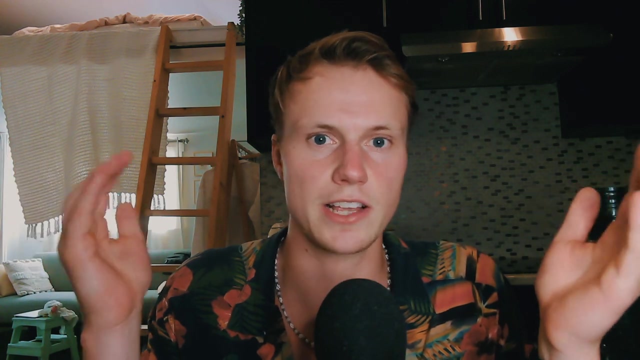 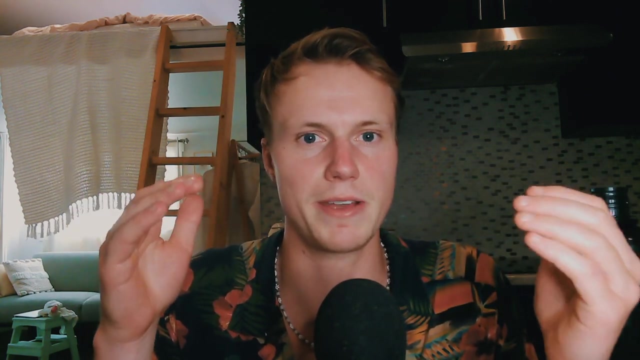 for that. we had a lot of issues with that, And so we actually figured out the solution that needed to be done about how we should be going every step in order to make sure that that schedule is effective as we work through the code. And another thing we found was that 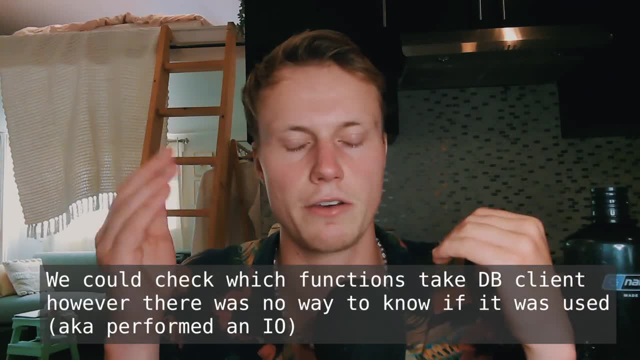 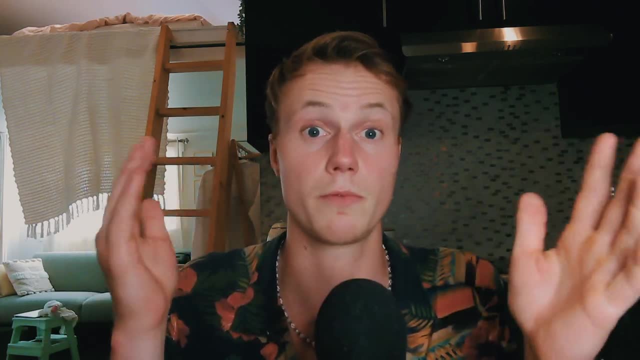 any way to make that referentially transparent, We had to kind of track down the variables and make sure that it's not getting passed around between the wrong functions. Now, obviously the project was written by like relatively new programmers, so I understood that this was going. 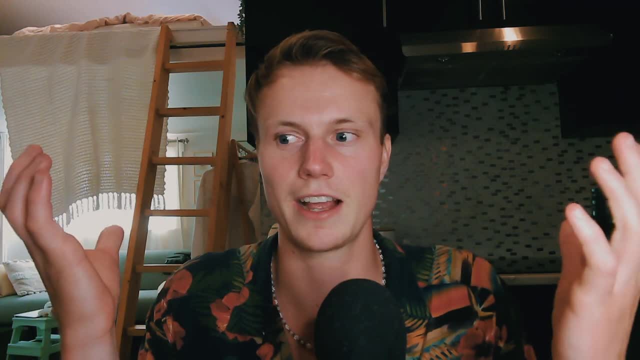 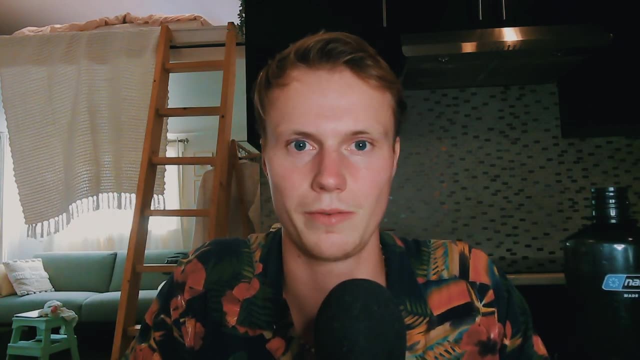 to happen, and it wasn't really something that I could prevent, besides doing excessive code reviews just all on my own, and so it became a huge issue. Now, this is kind of what sold me on Haskell- was the fact that debugging these issues when they came up would have been substantially easier if 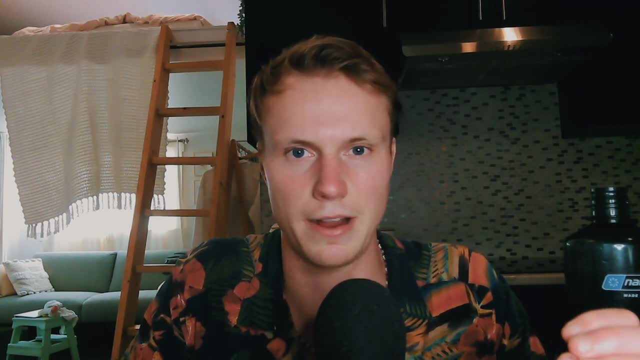 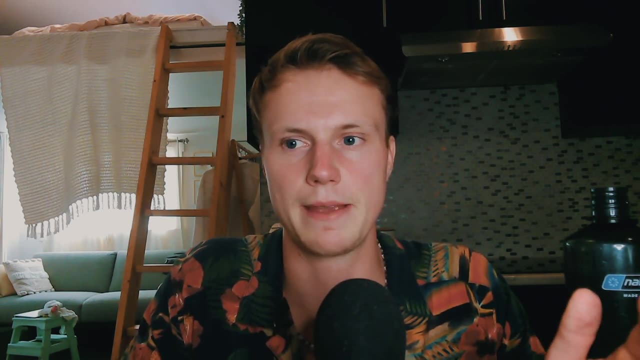 they ever came up, because it's a lot harder for them to come up in Haskell, because you have this referential transparency and you have very powerful primitives for doing these sort of concurrent actions, especially when it came to checking the Redis database and everything like that. It 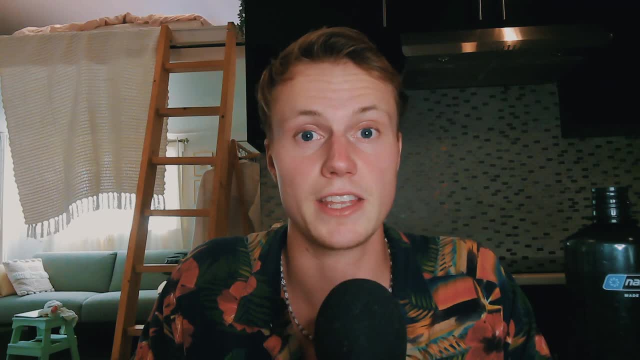 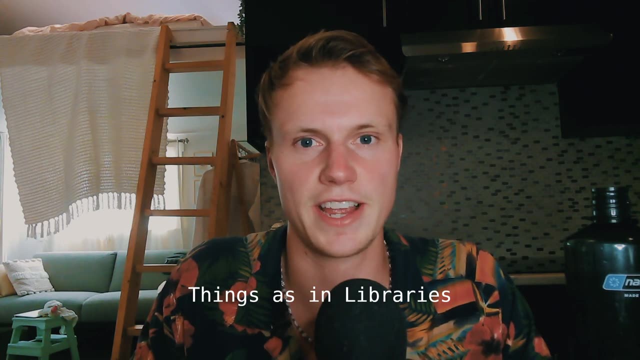 obviously is very intuitive with this. One of the greatest things about this is the fact that we didn't have to worry about things being thread safe if we used Haskell versus with Go. there was lots of edge cases where something wasn't quite thread safe and there wasn't really any way to know that it wasn't going to be thread. 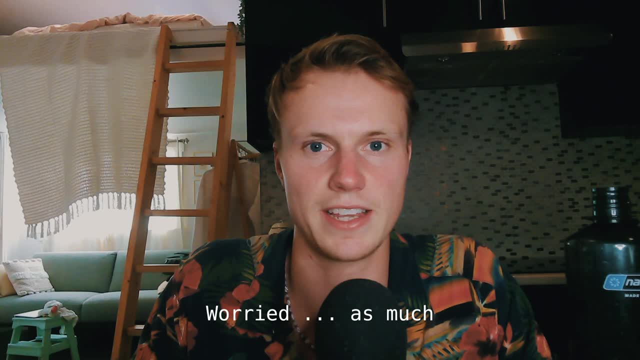 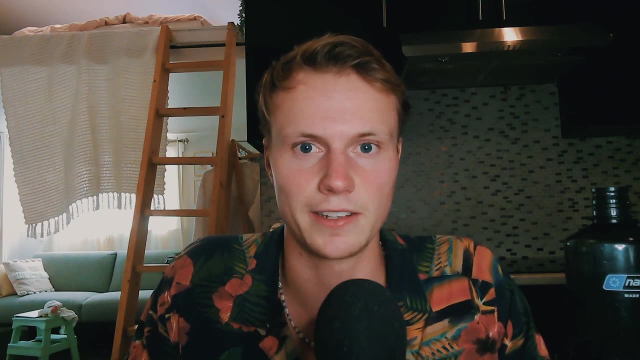 safe. If we had done this in Haskell, we wouldn't have to have worried about this and I wouldn't have spent quite as much time debugging when these edge cases would come up. Now, one of the big selling points that we get with Haskell is transactional memory. Now, I would have liked to 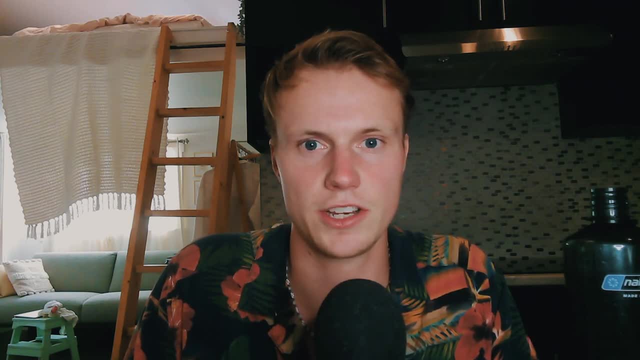 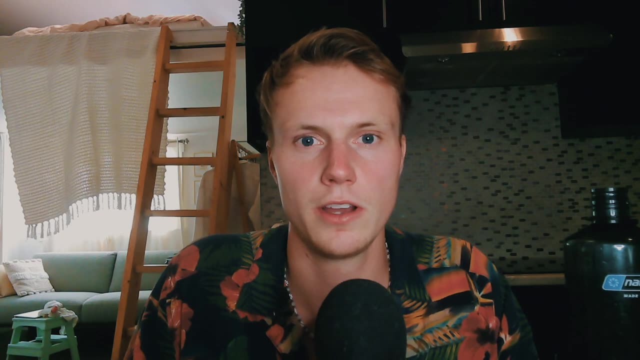 dig a bit more into transactional memory. but unfortunately, due to the shortage of time to make this video and kind of get this out to you, I've decided to cut it off and I'll put it in another video, although I will put something down in the description. 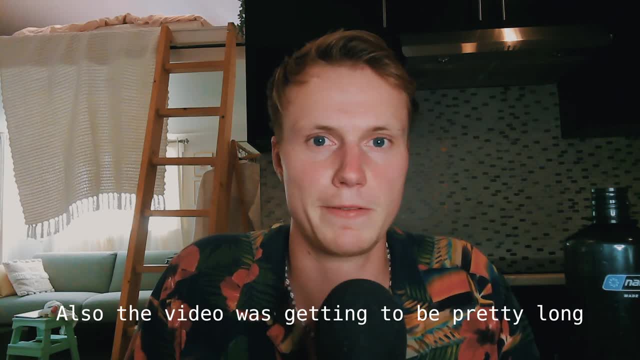 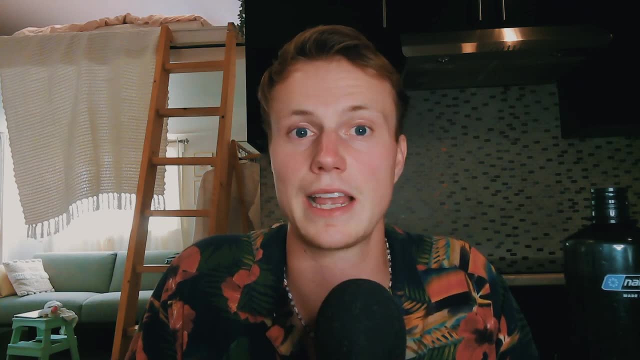 so you guys can kind of look into it. It's very powerful. the concept exists in other languages and as libraries, but Haskell probably is one of the things that does it the best, purely because of its language features. What exactly does the average developer get out of, even looking at? 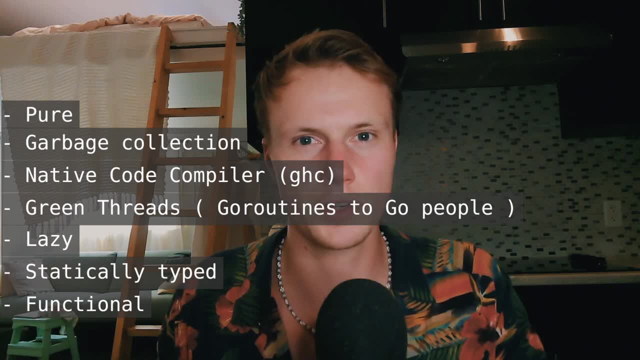 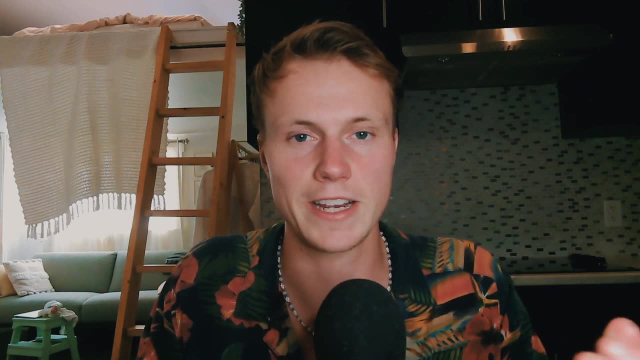 Haskell. Well, here's a really quick list of all the main go-to features of Haskell, and we talked about a lot more than just that in this video. Probably the biggest selling point, like I mentioned before, is its concurrency possibilities and prowess, as well as being able to compile. 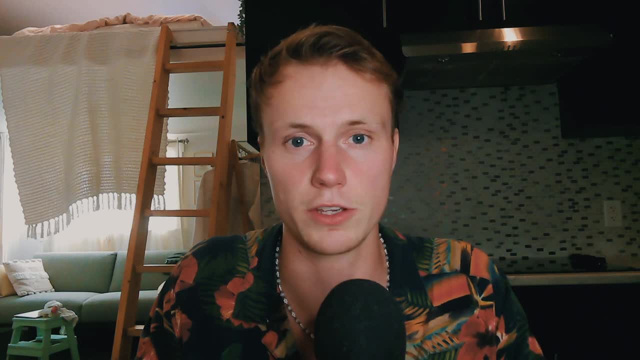 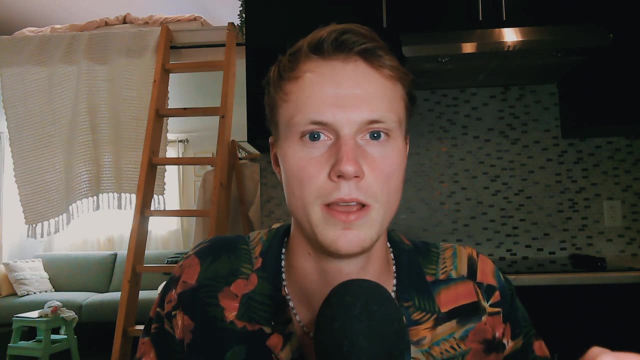 to a native executable and having garbage collection. it's a very powerful use case for the language, Especially for those of you coming from Rust who love the power that it offers you in the type system but want something a bit simpler for a concurrent code base where you 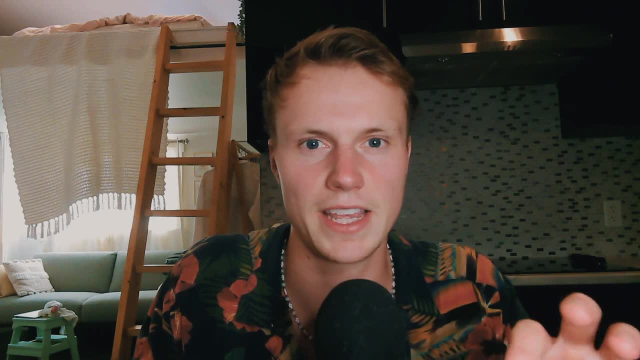 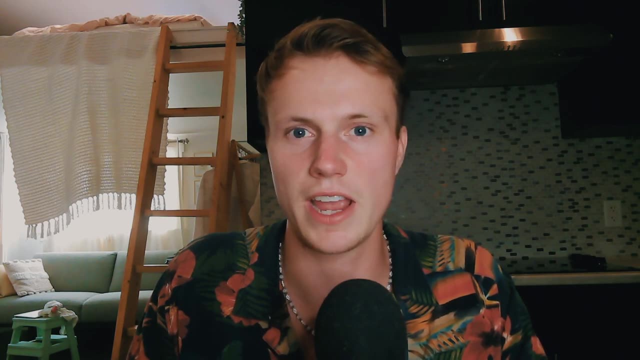 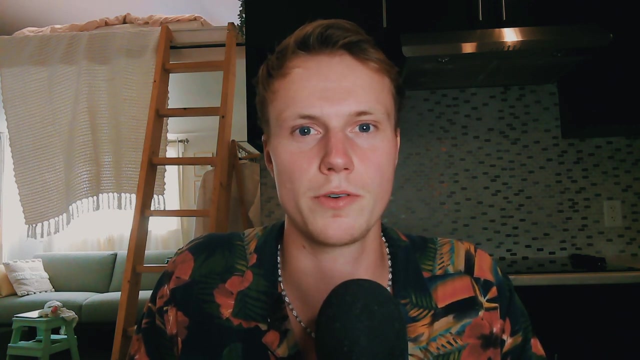 want garbage collection. you want a lot of the more finicky parts just dealt with for you. Haskell is a really powerful option there. Now, outside of the language functioning for a regular developer, I want to talk about what you can actually learn from writing Haskell. I feel like this has been beaten to death, but I do want to reiterate some of these thoughts that you 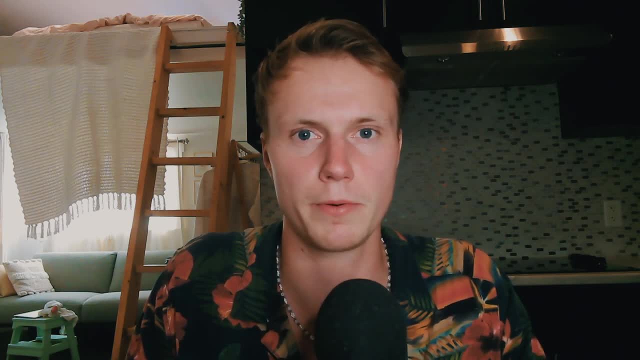 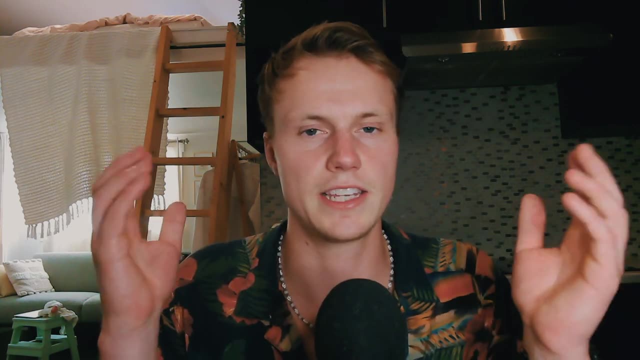 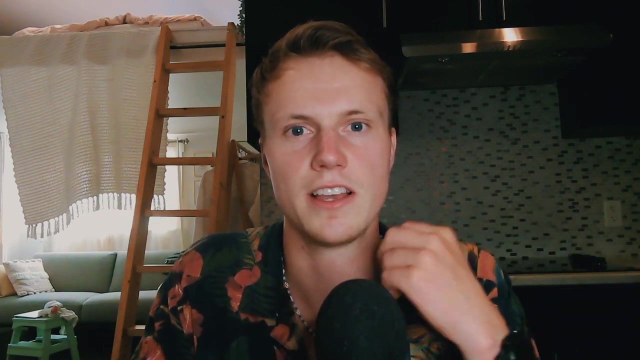 may have heard before, and that's how Haskell helps you become a better developer, even if you're not using Haskell. The big reason for this is really just the concept of the asynchronous code and the purity of the language. You kind of learn to be a bit more careful about how you use effects such as 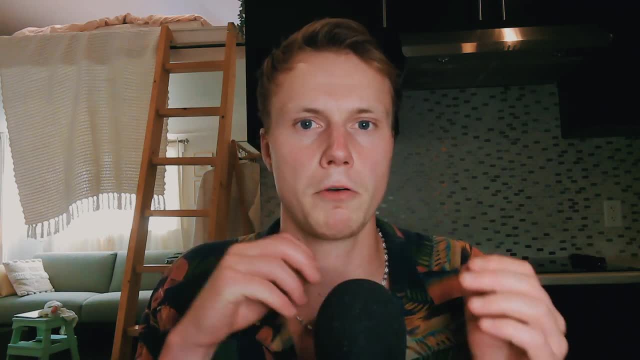 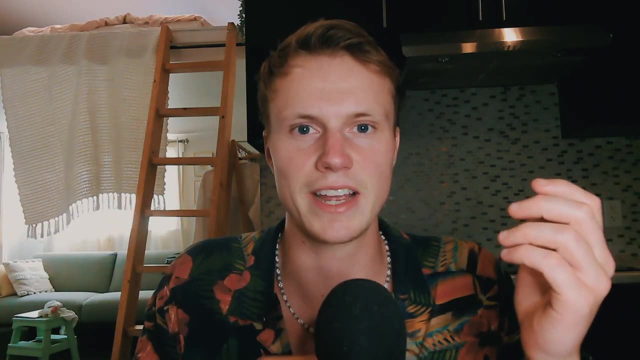 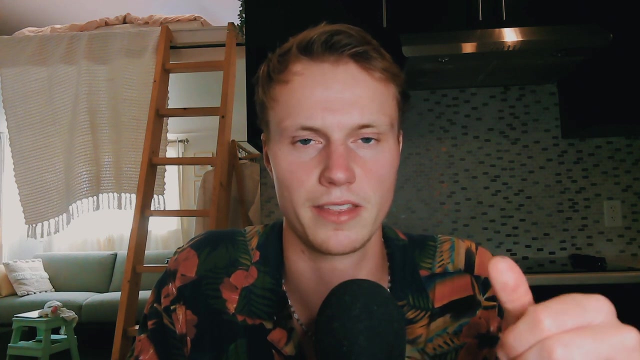 printing or manipulating a variable and you find ways to push them to the edge of your code base. This is really useful for people who design a lot of programs and for those of you who want to write nice, clean code with a pretty nice interface and very clean, easy, understandable systems that it works with. Now, while anyone can write a purely 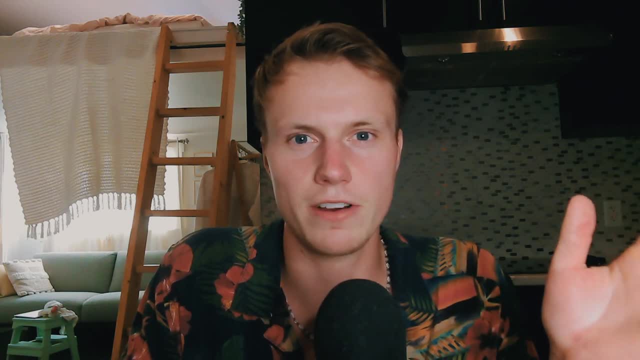 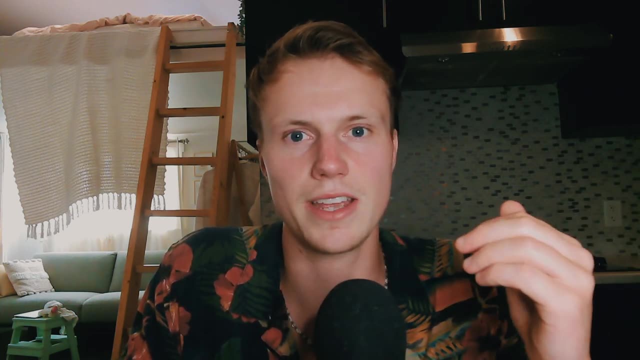 functional function like adding one and two. not everybody can design a system that makes good use of those effects, and this is kind of where I think Haskell really shines. It's less so in being able to write functions, because I think really a lot of things can be written quite easily without any. 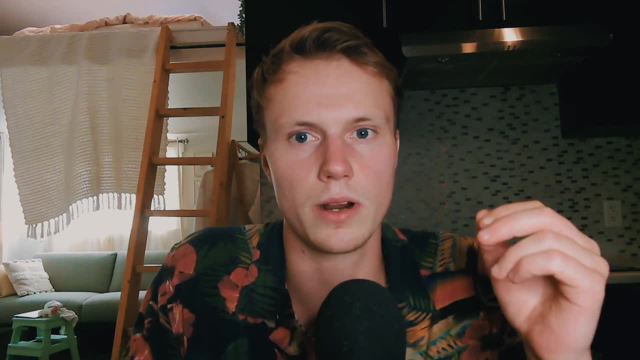 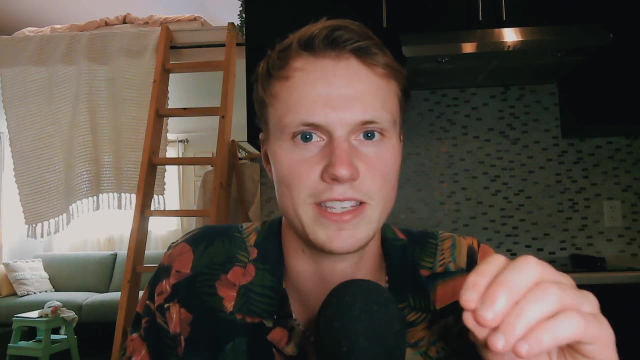 process and deal with these different effects like printing, or make your remote asynchronous request, and how to kind of encapsulate them to keep them from being a major part of your code base that everything has to kind of work through. It makes your code a ton easier to read because everything is all pure functions. you can read the input and output. you get 90% of what's going on. or you can even make your code more testable. you get a ton out of it, and so, while you don't have to become some crazy functional programmer, you do learn a ton from working with Haskell. 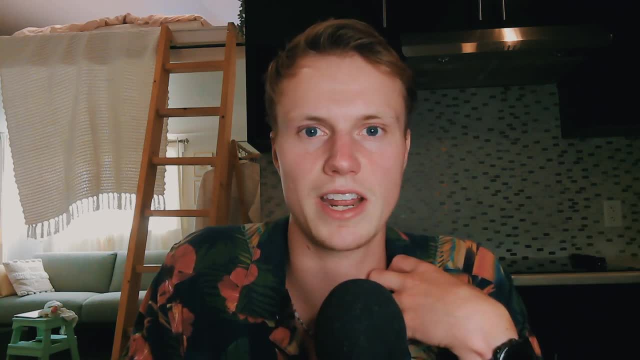 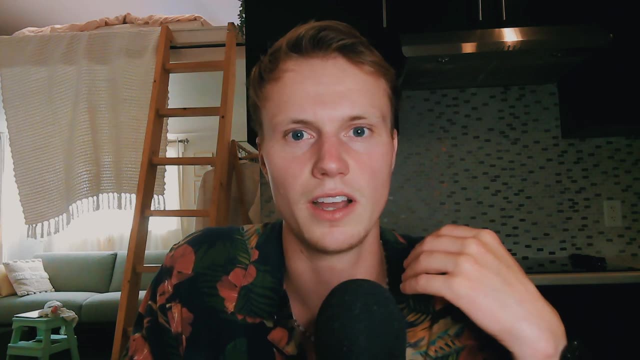 This is like a huge thing for me. you learn a lot about a concept, especially if you're not working with Haskell itself. you learn a lot about something called the functional core and then imperative- I forget what they call it. functional core, I know is like the big thing that they call.